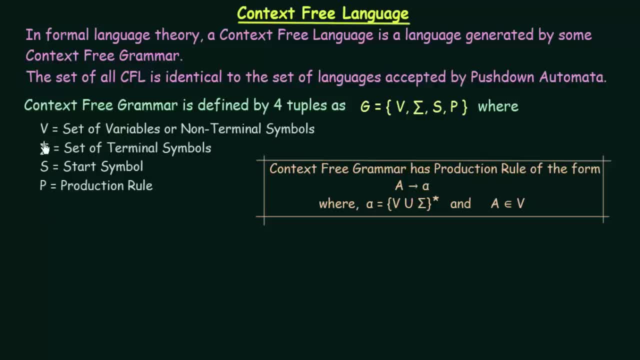 The tuples. actually, they mean the same as in the case of regular languages, where v is the set of variables or non-terminal symbols and sigma is the set of terminal symbols and s is a start symbol and p is a production rule. So what is the difference between regular grammar and context-free grammar? 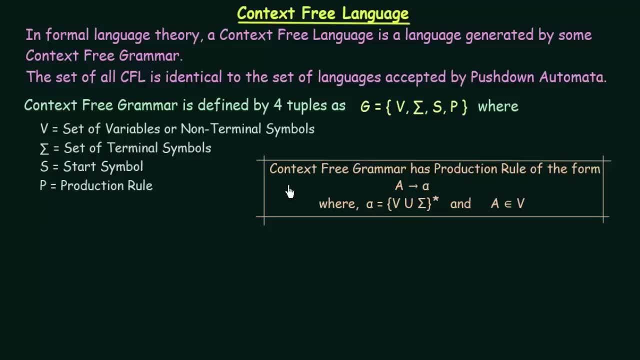 Actually the difference lies in the production rule. So in context-free grammar it has a production rule of the form a tends to alpha or a gives alpha, where alpha is the union of v and sigma closure. So that means that alpha can be a non-terminal symbol or a terminal symbol. 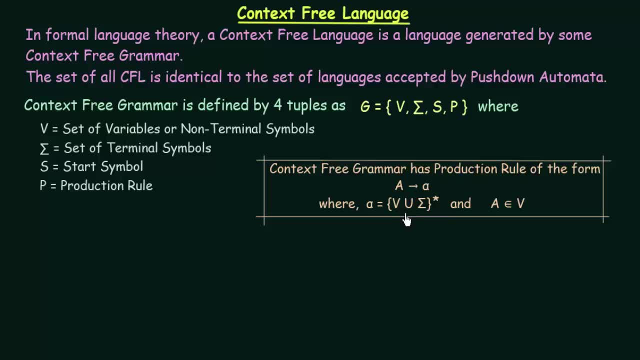 And here we notice that it is a closure, So that means that it could also be empty. It could also be an empty symbol or anything from a non-terminal symbol or a terminal symbol, And then a. It belongs to v. That means a belongs to the set of non-terminal symbols. 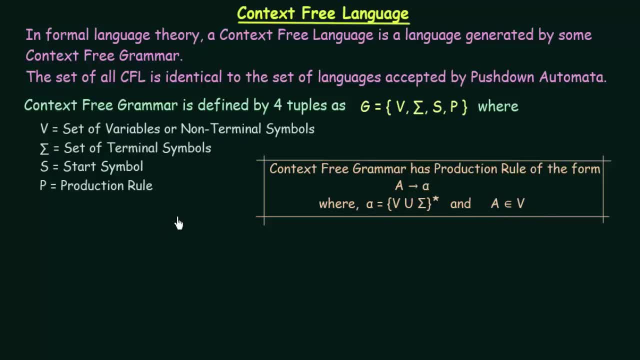 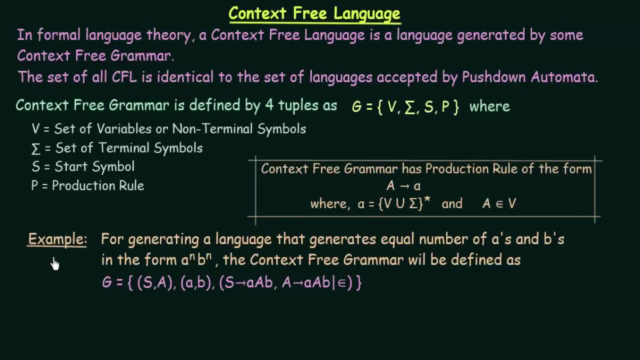 Okay, so this is how we formally define a context-free grammar. Now let us take a simple example to understand it in a better way. Alright, so here we have an example For generating a language that generates equal number of a's and b's in the form a power n, b power n. 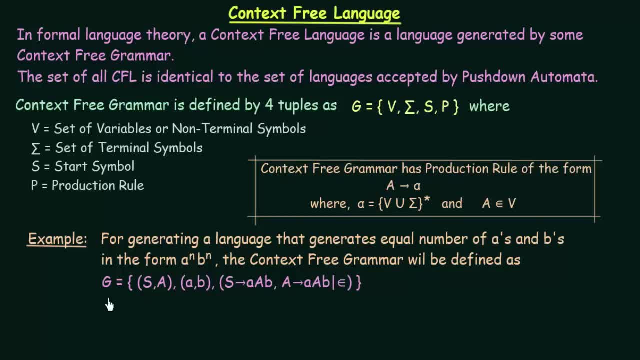 the context-free grammar will be defined as g equal to s, a, a, b, and this is a production rule. So, if you remember, we have taken this example a few times when we discuss regular languages And we already saw that this language, a language that generates strings of this form. 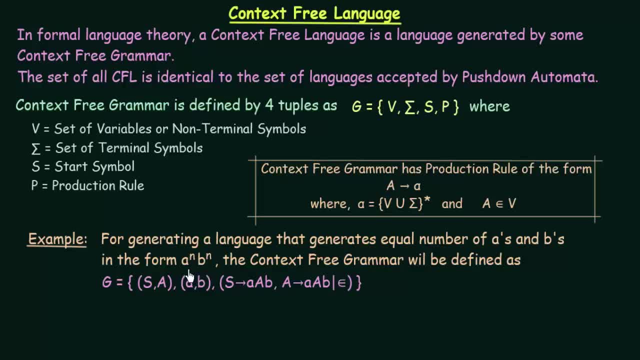 a power n, b power n, where the number of a's should be exactly equal to the number of b's, is not a regular language. And we already saw why it is not a regular language: Because this cannot be designed using a finite state machine. 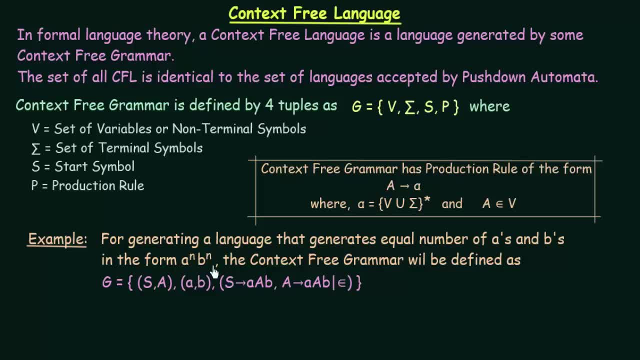 Since this could not be designed using a finite state machine, we are studying about context-free language now, And context-free language, as I told you, is a higher level of language as compared to regular languages, And context-free languages will be able to generate strings of this form. 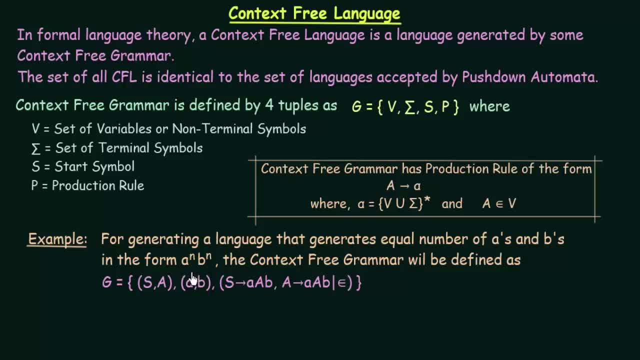 Okay, so we will see how this will be generated using context-free language. The grammar that will be used for generating this is defined like this: g, equal to s and a, which are the set of non-terminal symbols, And a and b are the set of terminal symbols. 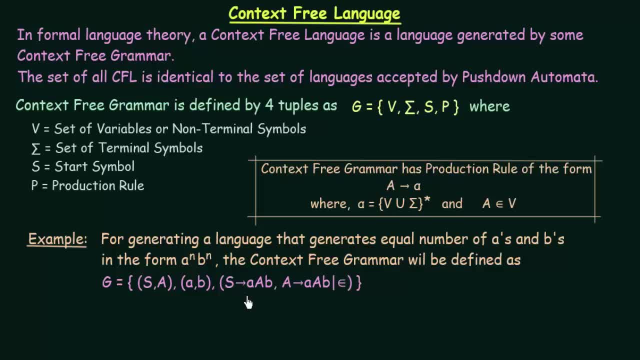 And we have a production rule of the form: s gives a a b and a gives a a b, and also it gives epsilon or the empty symbol. Okay, so here actually the start symbol is not given. So we should know that the start symbol is not given. 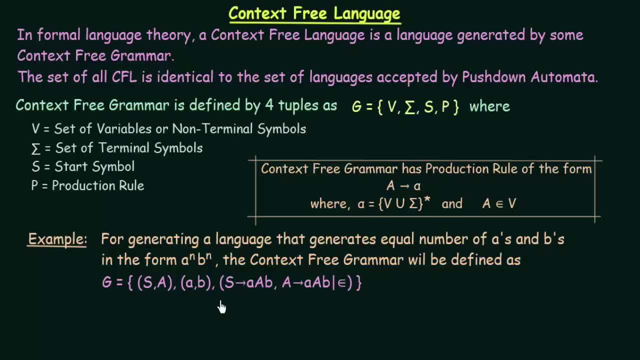 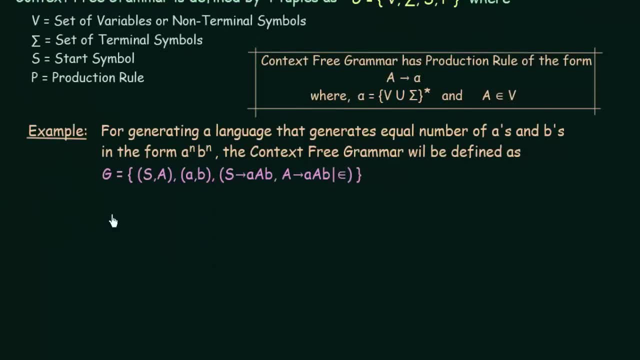 So we should know that the start symbol is not given. So, even if it is not given, let us understand that the start symbol is S over here. Okay, now let us see If this production rules will produce the string of this form. 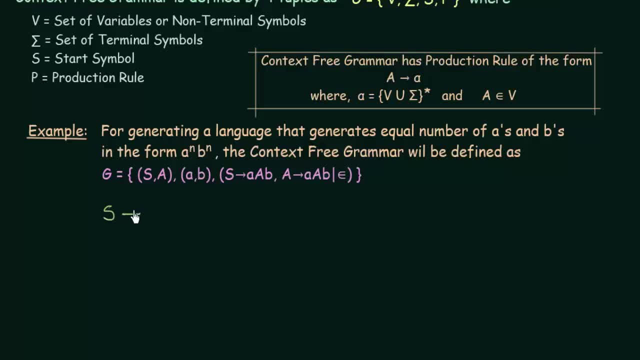 Okay, so let me start with my starting symbol, that is S, and S gives a a b. So, using this production, I have written this SGivesAB, another production rule, which says a gives a a b. so this a over here i will replace it with: 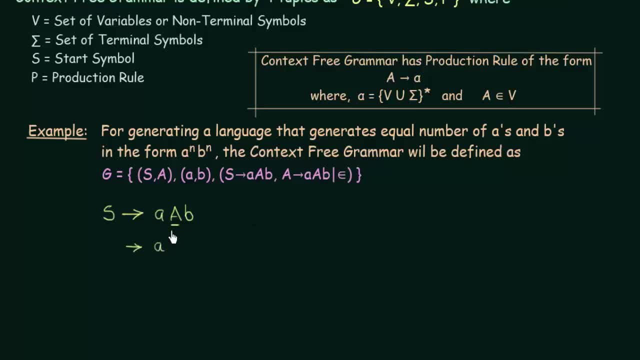 a, a, b. so this a will come down as it is and this capital letter a will be replaced by a, a, b, a, a, b and this b over here comes down as it is. so this is by the production which says a gives a, a b. all right, and now let's try to expand this further. here we have a, a, a, b, b. now this a. 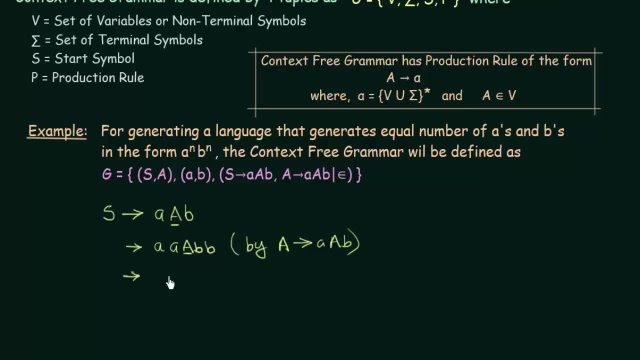 using the same production rule. i will expand it again, so these two a's will come down as they are, and instead of this a, i will write a, a, b, a, a, b, and these two b's are remaining. they will come down as they are. so this is also using the same production rule as above. 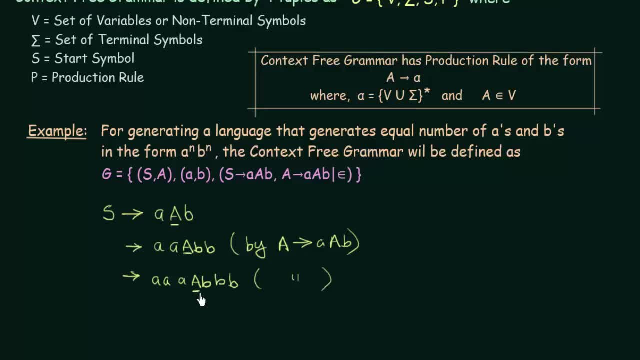 okay, you now i still have a a, which is a non-terminal symbol here and now what i will do is i will replace this a with epsilon, that is, the empty symbol, because we see that the production rule says a gives a, a, b, and also it can give epsilon or the empty symbol. so i can write a, a, a and